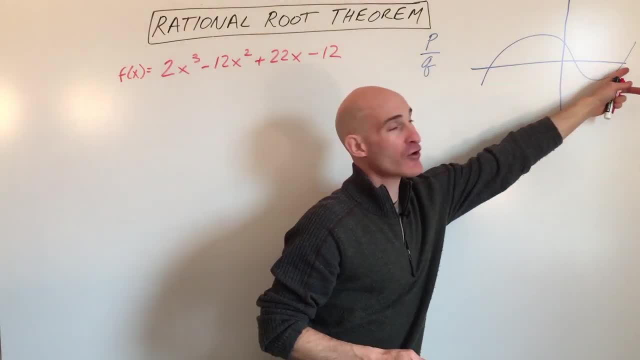 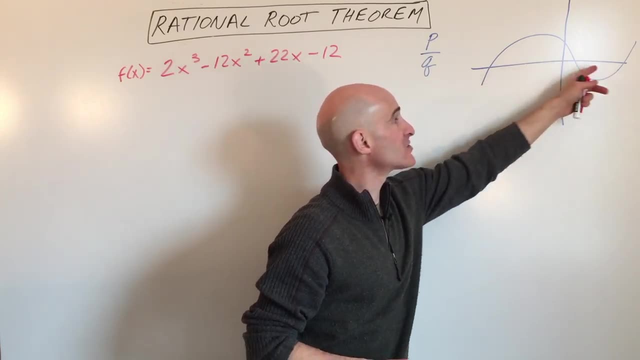 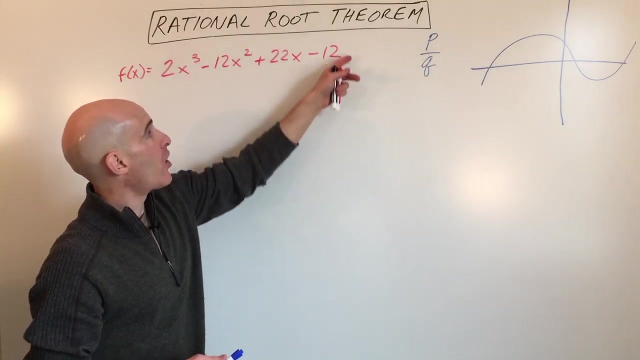 to zero, And these are also the points where the graph crosses the x-axis. So that's the roots. okay, they call these roots solutions, x-intercepts, zeros- those all mean the same thing, And so the way we find these rational roots is by taking all the factors of the 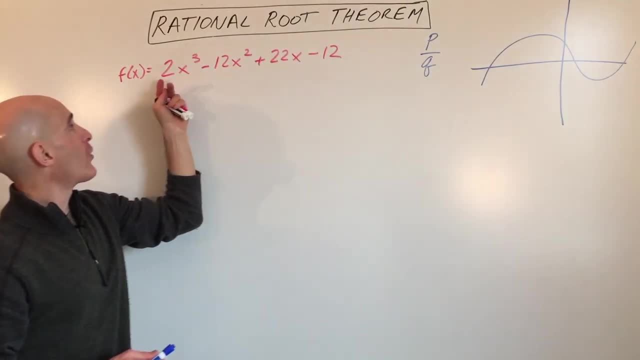 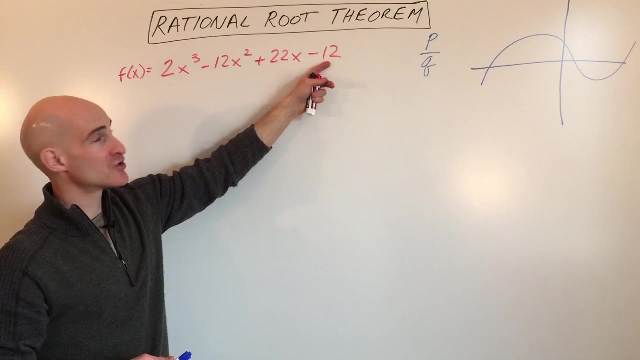 constant- sometimes we refer to that as p- over all the factors of the leading coefficient, this number here in front. So all the factors of the constant meaning, all the numbers that divide in evenly to 12, all the integers divided by all the integers that divide in. 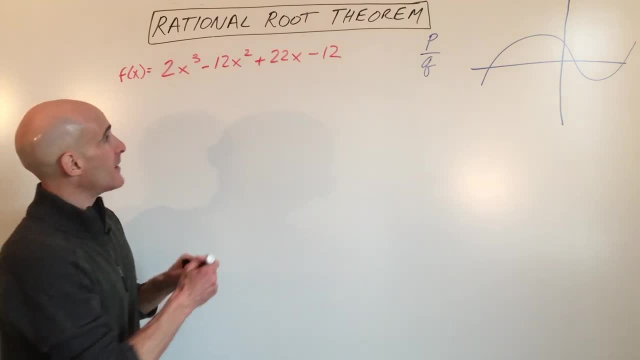 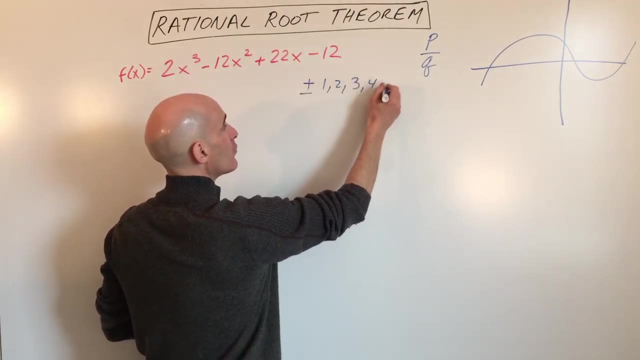 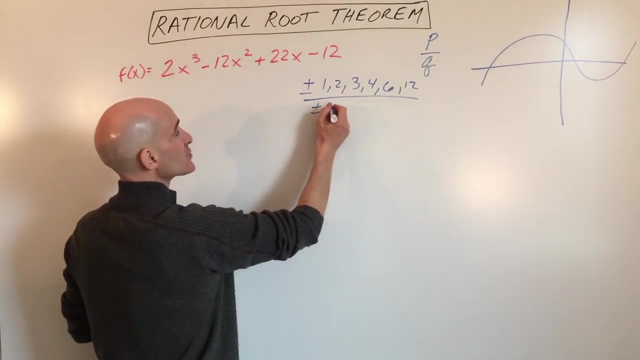 evenly into this leading coefficient, 2.. So if we're going to do that, all the factors of 12 are going to be plus or minus 1,, 2,, 3.. 3,, 4,, 6, and 12. And all the factors of the leading coefficient would just be plus or 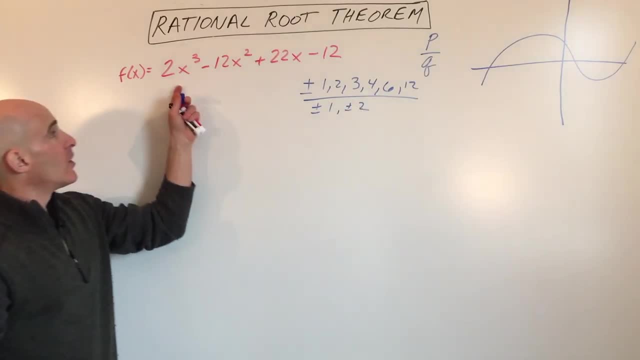 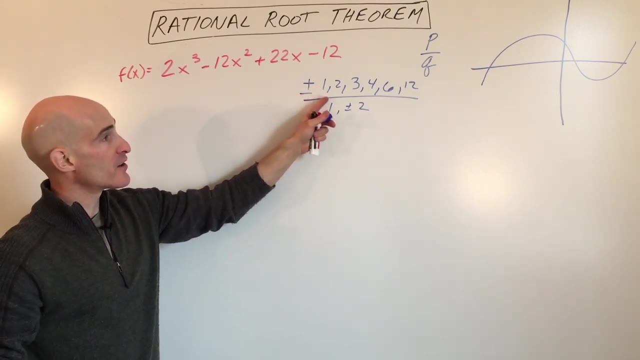 minus 1 or plus or minus 2.. So these are all the numbers that divide in evenly to the leading coefficient. So now what you can do is you can take any number in the numerator divided by any number in the denominator and come up with a possible rational root. So these 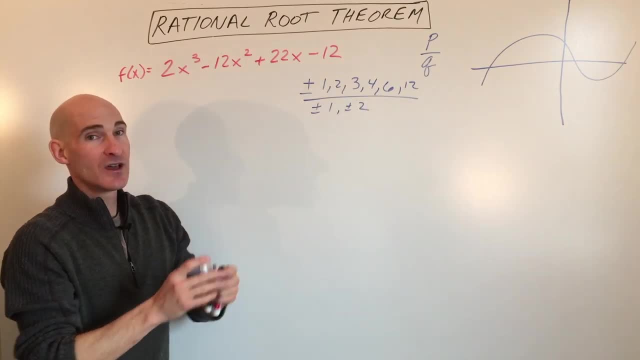 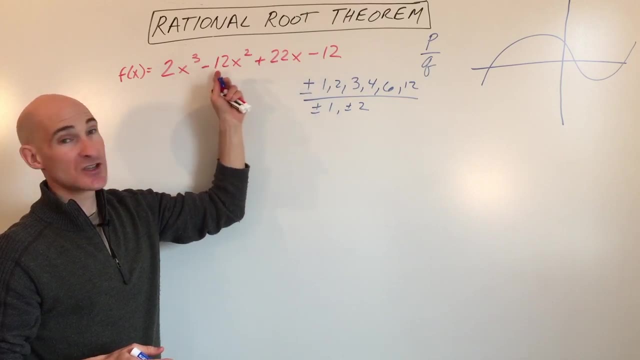 aren't guaranteed to be the roots, but what it does is it narrows down. uh, you know the possibilities that you could try in order to find out. you know a root or a solution or a zero of this polynomial, So you're narrowing down Like if I had to. you know, guess which? 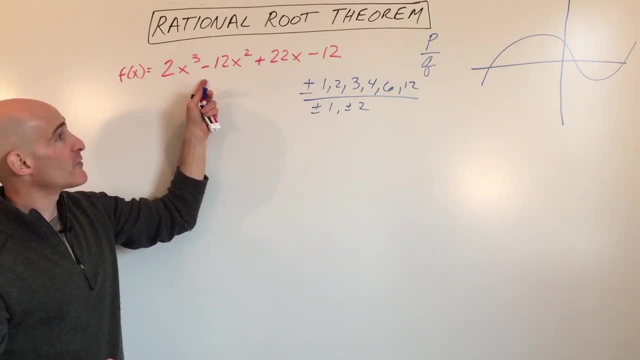 number would make this equal to zero. it might be a while for me guessing. I might try and factor this and set the factors to zero, but it might not be easily factored. It might not be in a form that I recognize, And that's where the rational root theorem comes in. 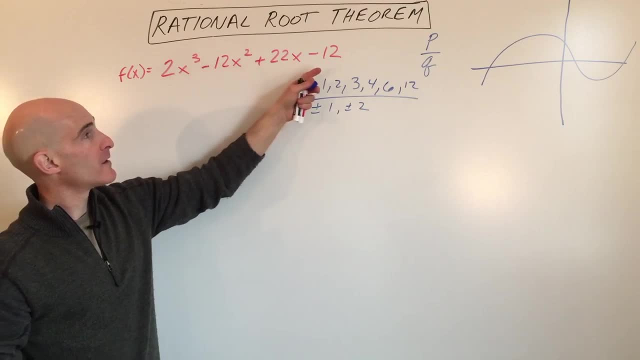 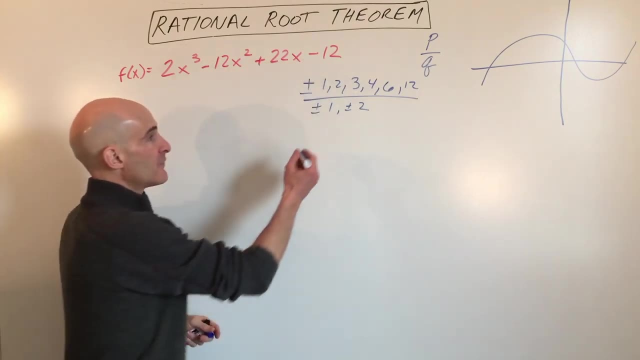 You can see, this isn't a quadratic, it's a cubic, So it's a little bit more challenging to factor. So here's what we do: We take the factors of the constant over the factors of the leading coefficient And, if you want, you can write these out. You could say like this is going. 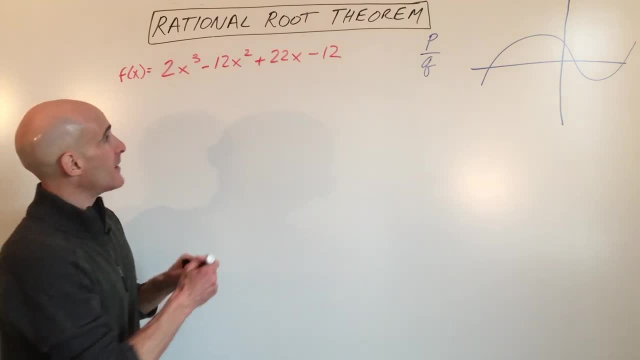 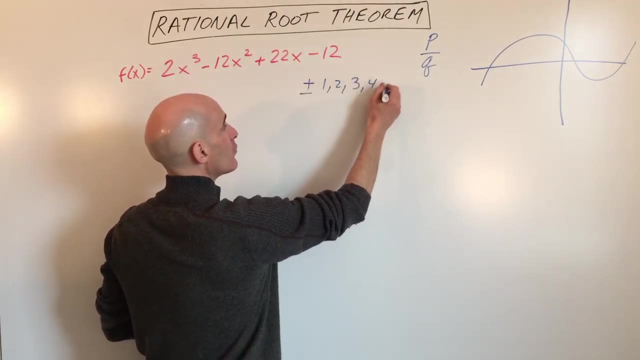 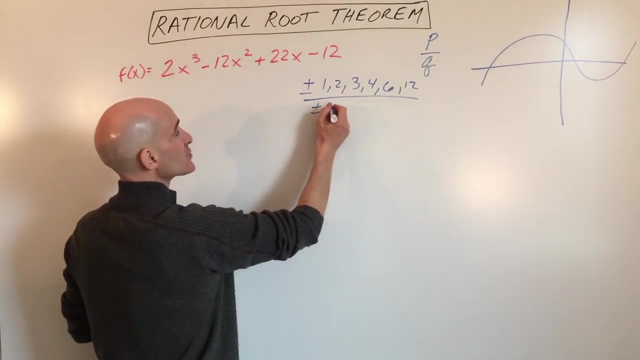 evenly into this leading coefficient, 2.. So if we're going to do that, all the factors of 12 are going to be plus or minus 1,, 2,, 3.. 3,, 4,, 6, and 12. And all the factors of the leading coefficient would just be plus or 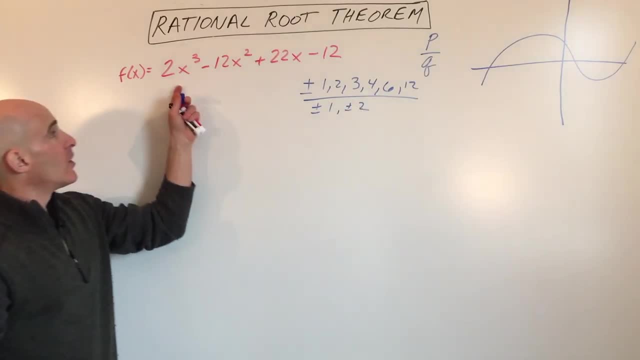 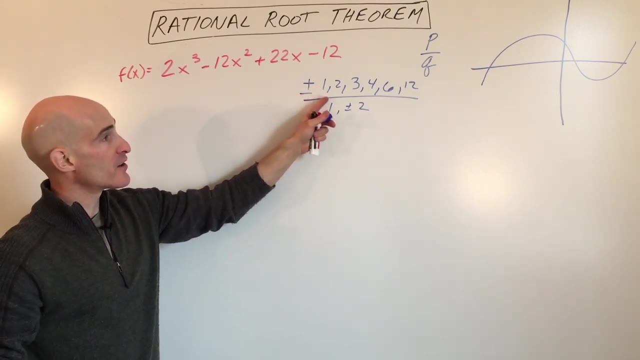 minus 1 or plus or minus 2.. So these are all the numbers that divide in evenly to the leading coefficient. So now what you can do is you can take any number in the numerator divided by any number in the denominator and come up with a possible rational root. So these 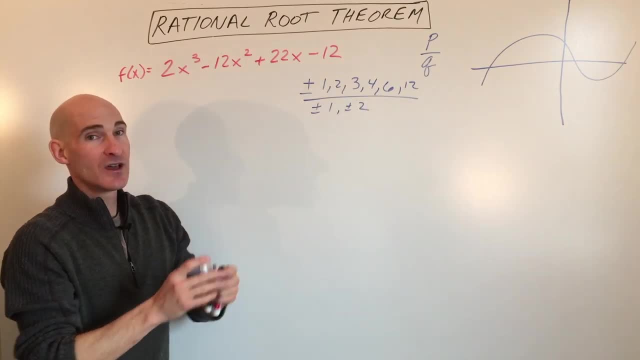 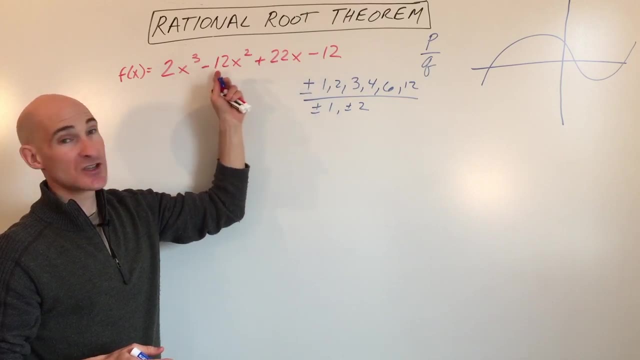 aren't guaranteed to be the roots, but what it does is it narrows down. uh, you know the possibilities that you could try in order to find out. you know a root or a solution or a zero of this polynomial, So you're narrowing down Like if I had to. you know, guess which? 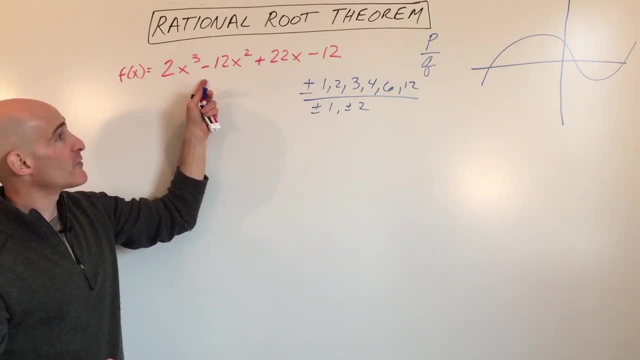 number would make this equal to zero. it might be a while for me guessing. I might try and factor this and set the factors to zero, but it might not be easily factored. It might not be in a form that I recognize, And that's where the rational root theorem comes in. 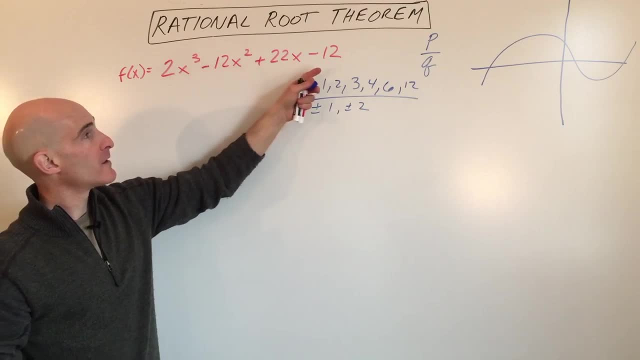 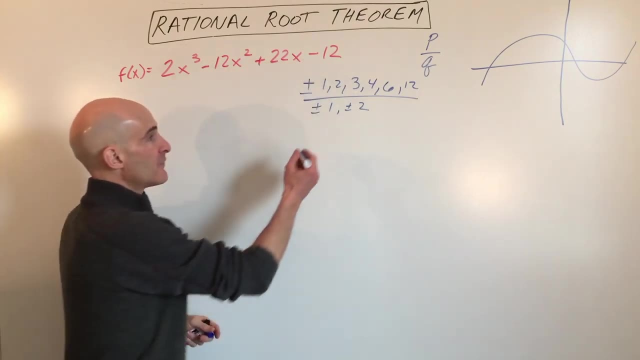 You can see, this isn't a quadratic, it's a cubic, So it's a little bit more challenging to factor. So here's what we do: We take the factors of the constant over the factors of the leading coefficient And, if you want, you can write these out. You could say like this is going. 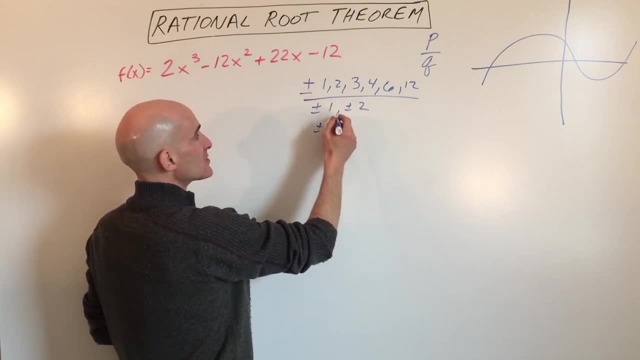 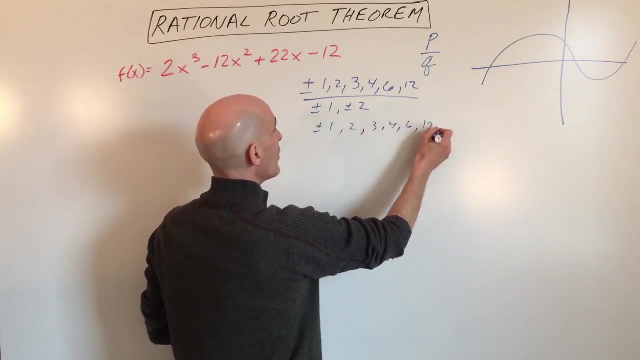 to be plus or minus, one over one, which is one. This is going to be two over one, which is two, So these all could be positive or negative. Three, four, six, twelve, Or it could be one half, Okay, so I'll just slip in one half right there, Okay, Or it could. 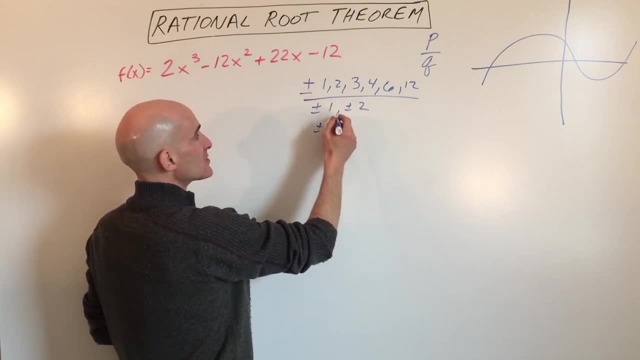 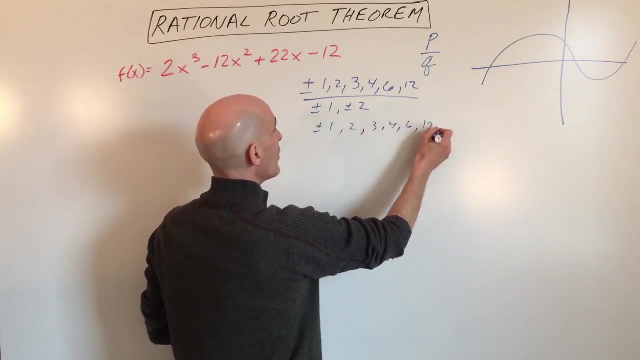 to be plus or minus, one over one, which is one. This is going to be two over one, which is two, So these all could be positive or negative. Three, four, six, twelve, Or it could be one half, Okay, so I'll just slip in one half right there, Okay, Or it could. 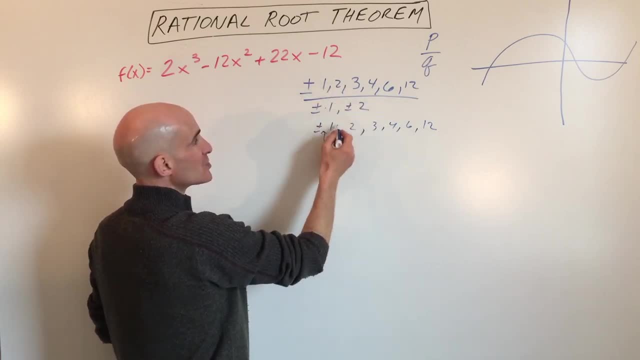 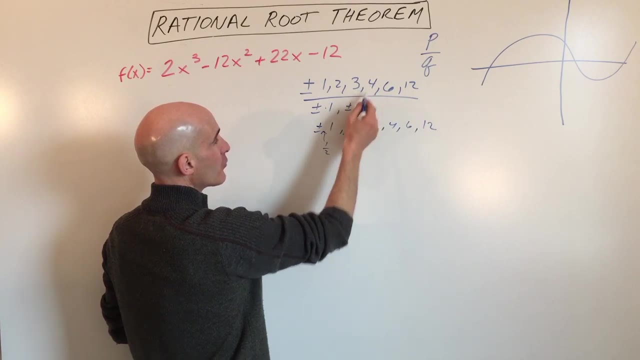 be two over one, which is two. we already have listed Two over two, which is one. Three over two. Okay, we don't have that one. I'll put that one in: Three over two. Four over one. We have that. Four over two is two. we have that Six over. 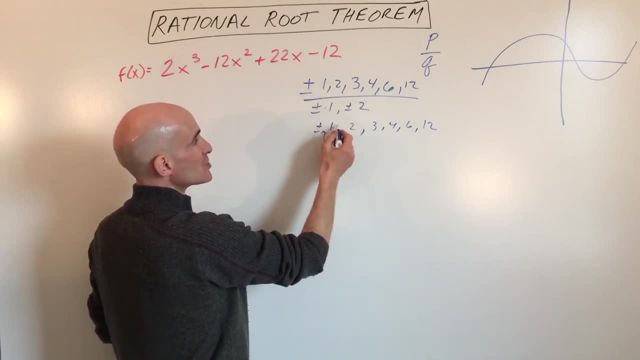 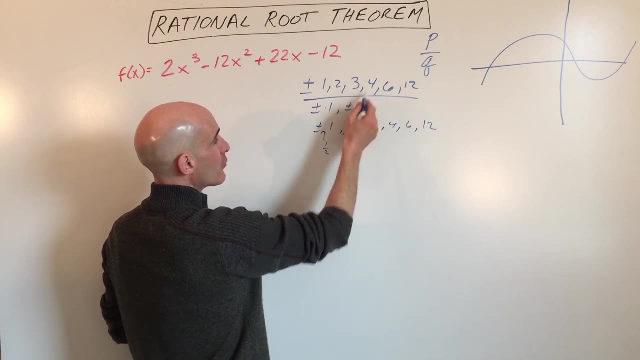 be two over one, which is two. we already have listed Two over two, which is one. Three over two. Okay, we don't have that one. I'll put that one in: Three over two, Four over one. we have that. Four over two is two. we have that Six over. 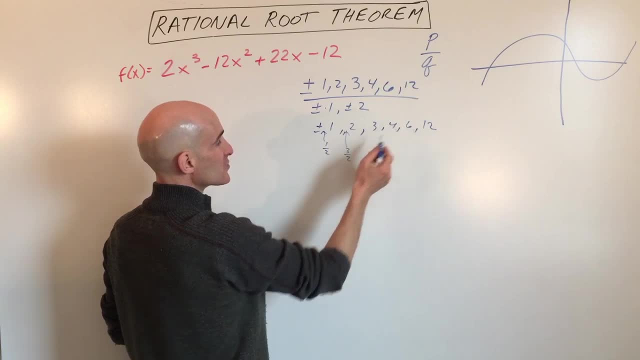 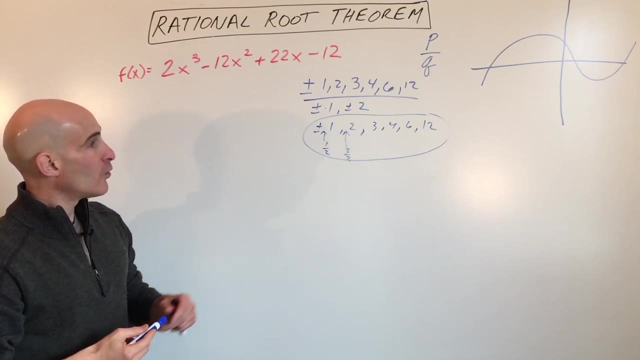 two is three. Six over one: we have that. Twelve over two, which is six: we have that. So these are all the possible rational roots. Now what we do to test them out is we do synthetic division. So let's say we wanted to test to. 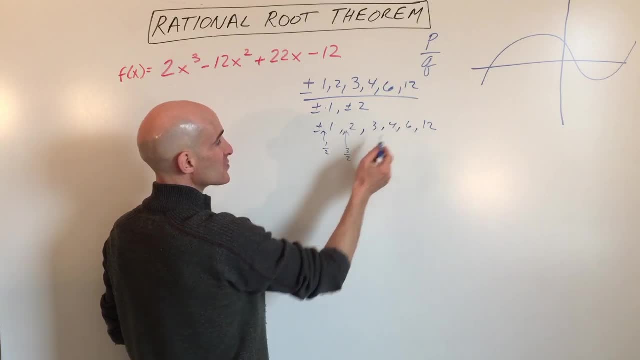 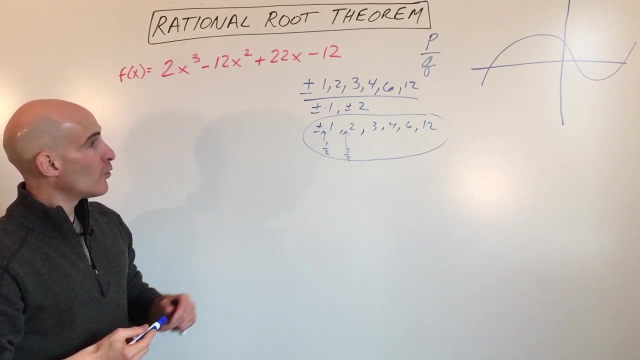 two is three. Six over one: we have that. Twelve over two, which is six: we have that. So these are all the possible rational roots. Now what we do to test them out is we do synthetic division. So let's say we wanted to test to. 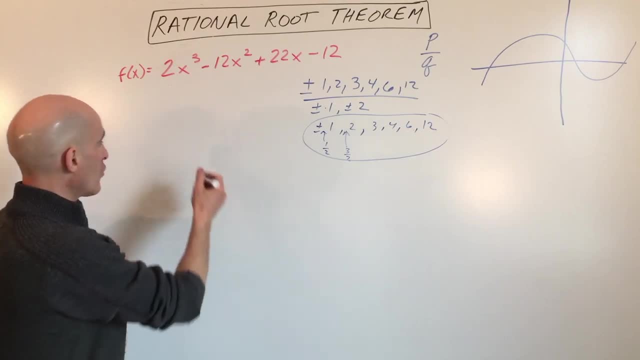 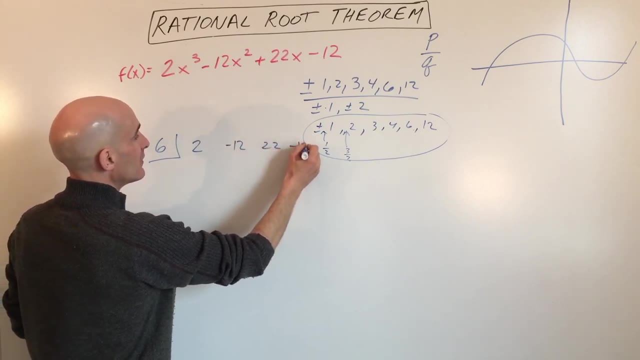 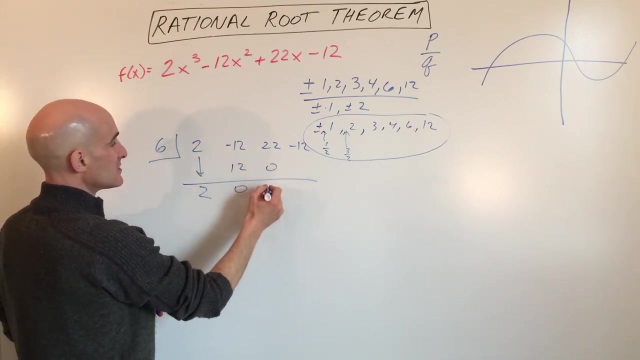 see if six was a root. What we do is we go over here and we do our synthetic division- Negative twelve, twenty-two and negative twelve, And we do our synthetic division. So this is twelve zero zero. twenty-two hundred twenty hundred thirty-two hundred. 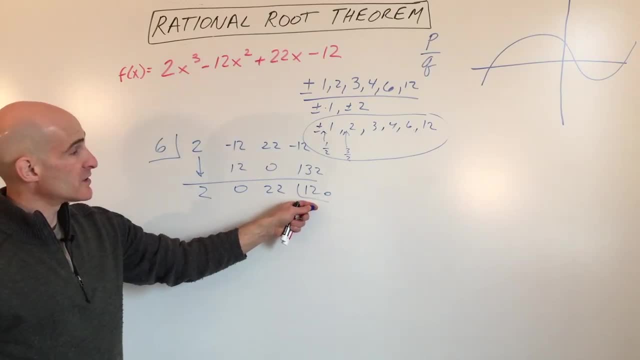 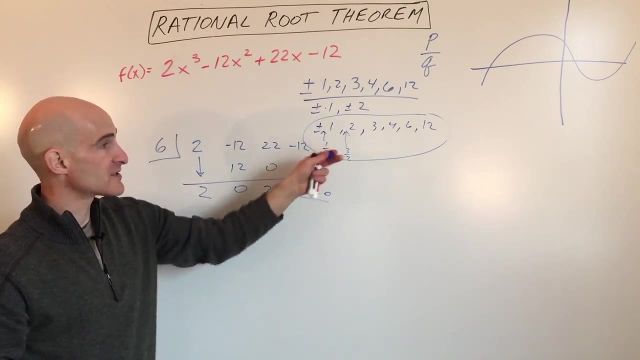 and twenty. So this one didn't come out to zero. So that means that six is not a zero, It's not a root of this polynomial. Okay, so cross that one off the list. Let's try another one. Let's say we want to try one. 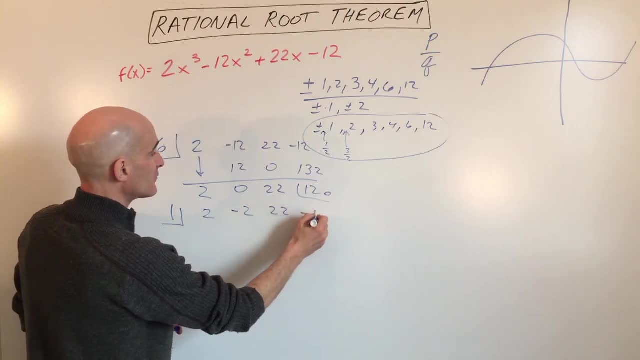 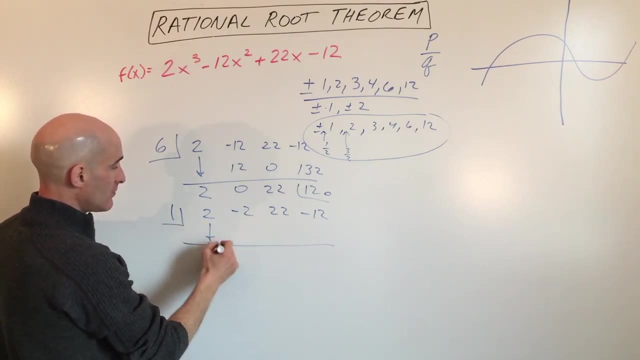 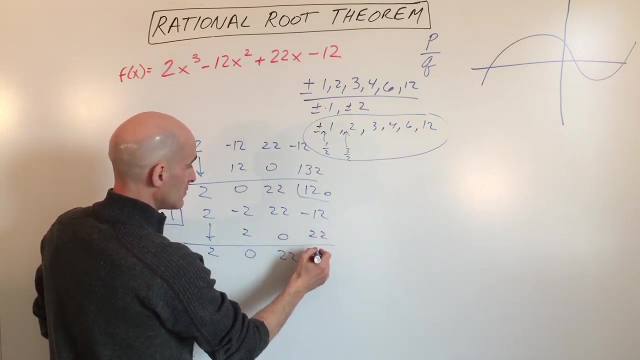 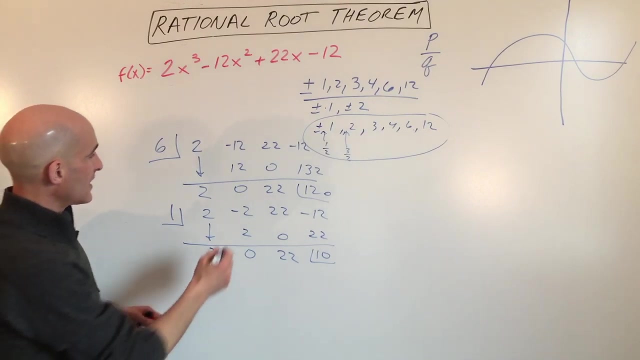 Okay, so two negative, two, twenty-two negative, twelve. Those are our coefficients. We're doing the synthetic division Two. two zero, zero, twenty-two, twenty-two, Okay, and this comes out to ten. So, oh, I made a mistake because this is twelve. Okay, let's do that. 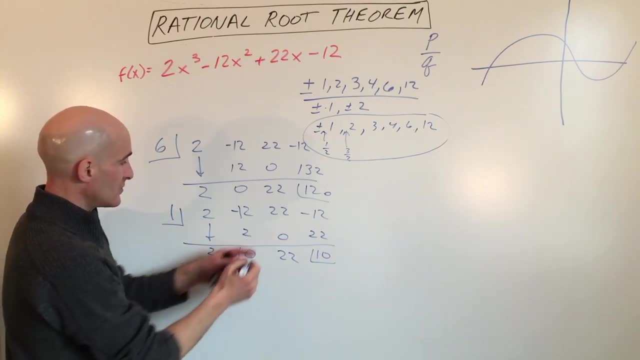 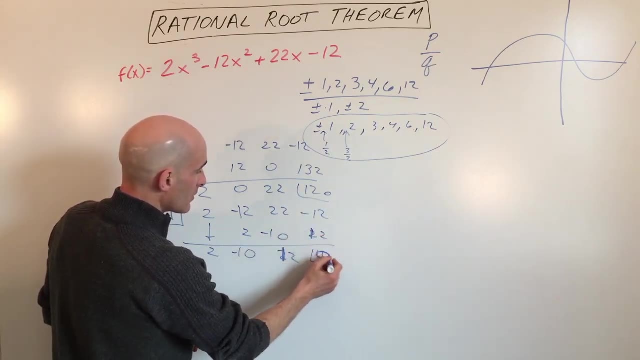 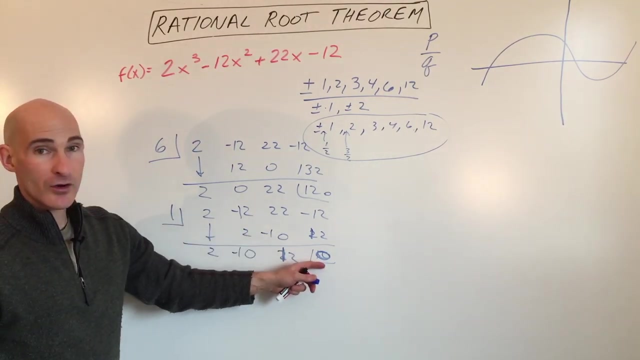 again. So this would be negative ten, This would be negative ten, This would be twelve, And then this would be twelve And this would be zero. Okay, so there we go. So we've got zero as a remainder. So that means that one is a zero. Okay, it is a root. And what happens? 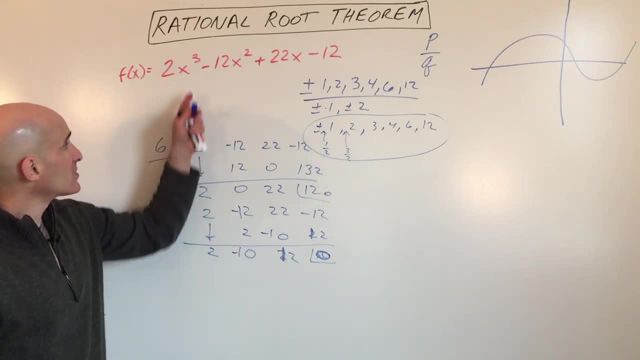 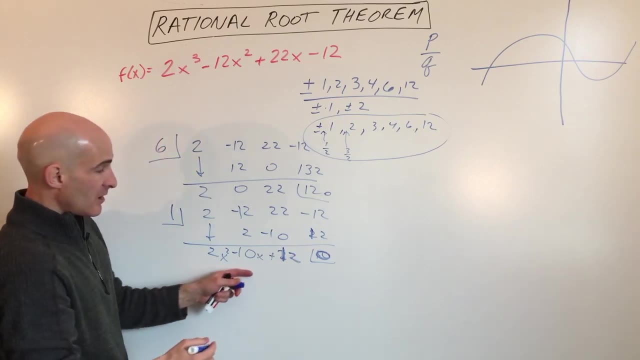 when you do the synthetic division is. this goes down by one degree. So originally it was a cubic, Now we're going to be down to a quadratic. So two x squared minus ten x plus twelve, And in quadratic we can do the quadratic formula to find the other zeros, or we can factor. 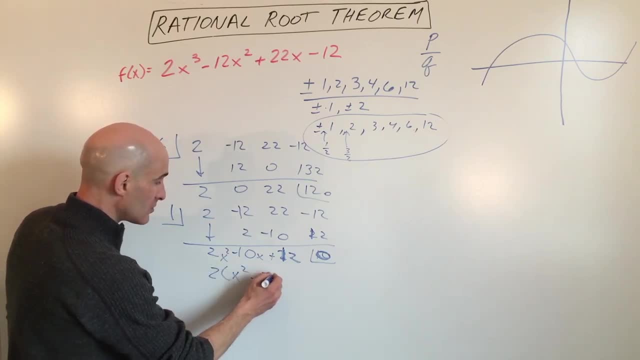 So here I'm just going to factor, I'm going to factor out the two, And here I can factor this into two binomials: X minus three and x minus two. If I set these factors equal to zero, we get three or two. Okay, so we have our zeros: One, two and three. Okay. 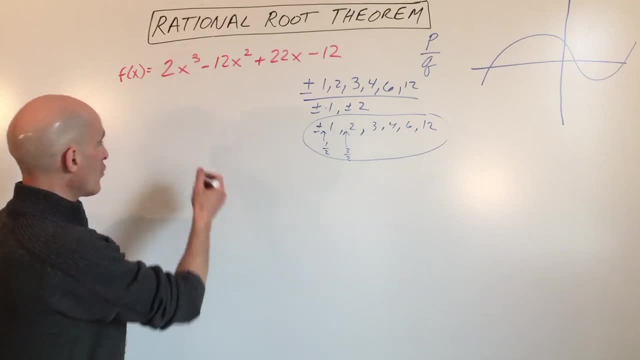 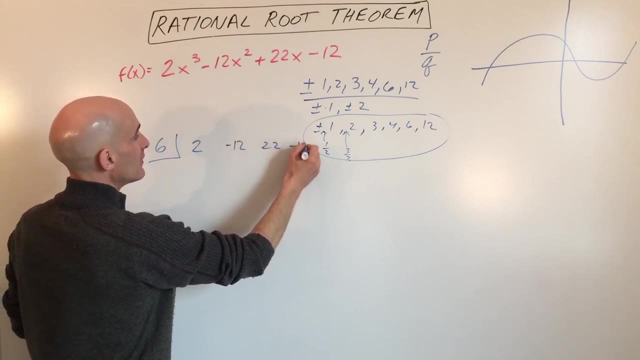 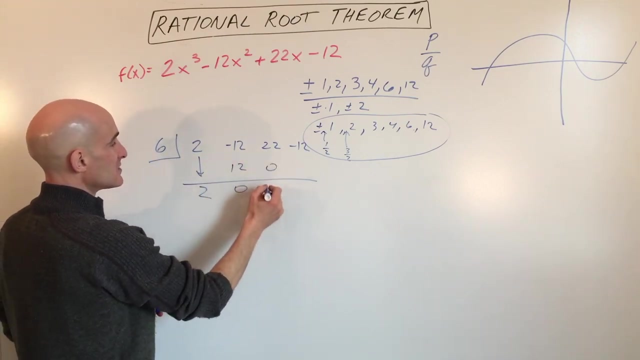 see if six was a root. What we do is we go over here and we do our synthetic division: Two negative, Negative twelve twenty-two and negative twelve, And we do our synthetic division. So this is twelve zero, zero, twenty-two, hundred-twenty, hundred-thirty-two, hundred-and-twenty. 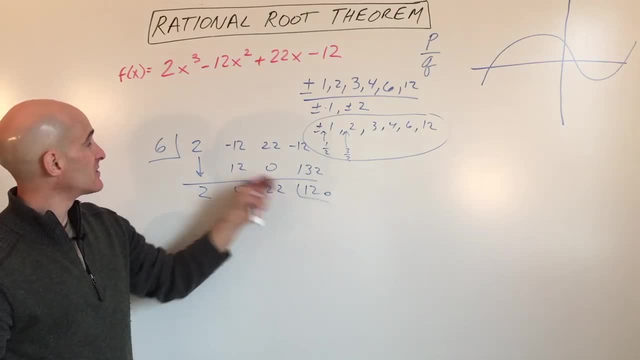 So this one didn't come out to zero. So that means that six is not a zero. It's not a root of this polynomial. Okay, so cross that one off the list. Let's try another one. Let's say we want to try one. 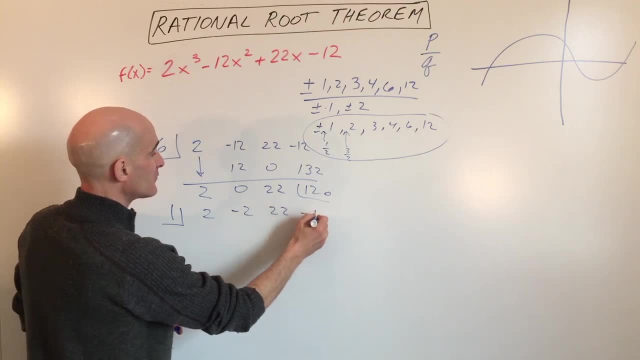 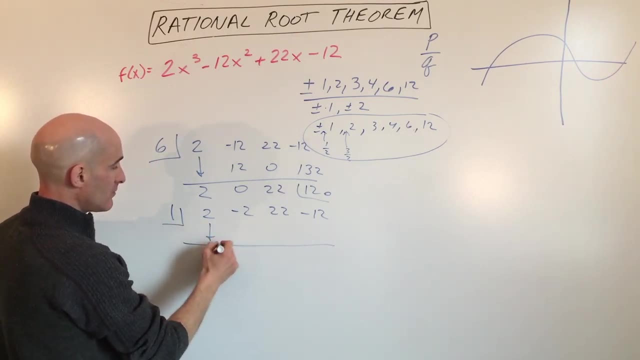 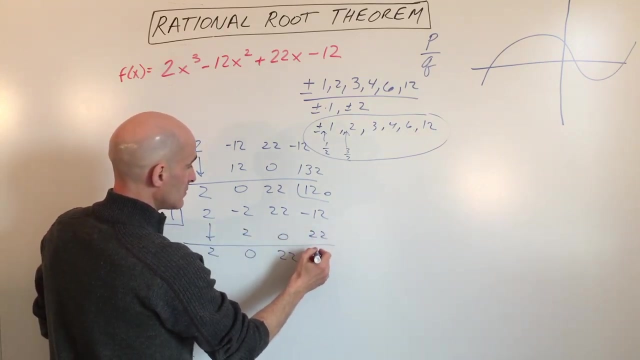 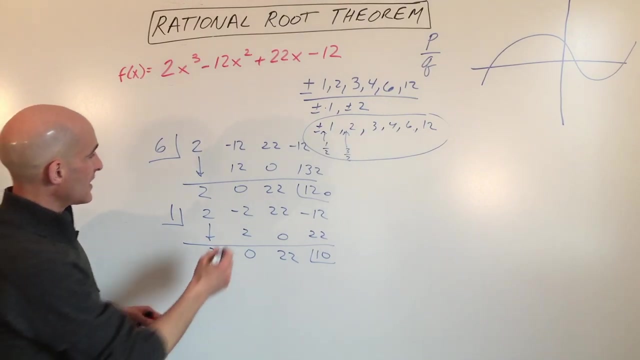 Okay. so two negative, two twenty-two negative, twelve. Those are our coefficients. We're doing a synthetic division: Two zero, zero, twenty-two, twenty-two, Okay, And this comes out to ten. So, Oh, I made a mistake, because this is twelve. Okay, let's do that again. So this: 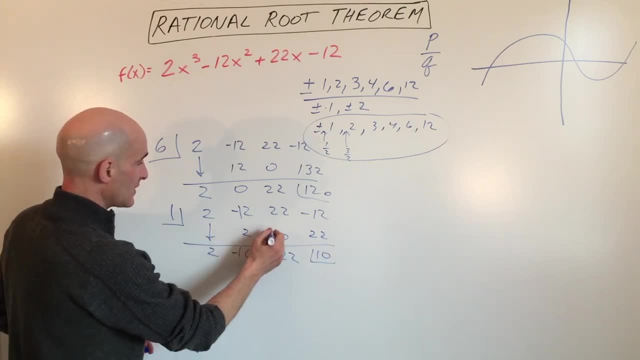 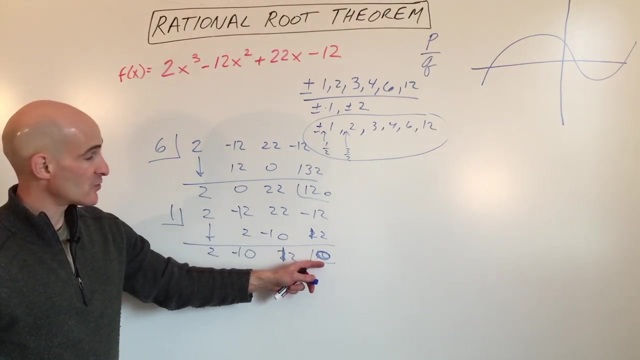 would be negative ten, This would be negative twenty-two, twenty-two, and this would be would be negative 10, this would be 12, and then this would be 12, and this would be 0. okay, so there we go, so that we got 0 as a remainder. so that means that 1 is a 0. okay, it is a root, and 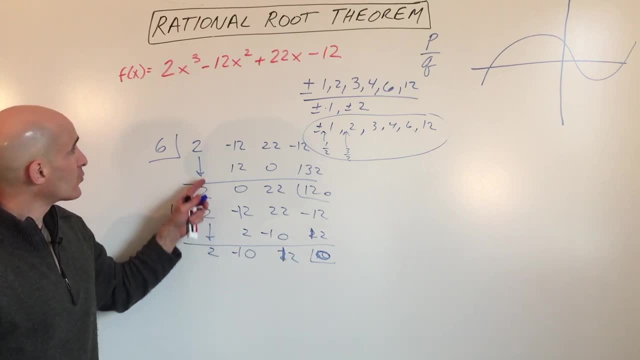 what happens when you do the synthetic division is: this goes down by one degree. so originally it was a cubic, now we're going to be down to a quadratic. so 2x squared minus 10x plus 12. now that it's in the quadratic we can do the quadratic formula to find the other zeros. 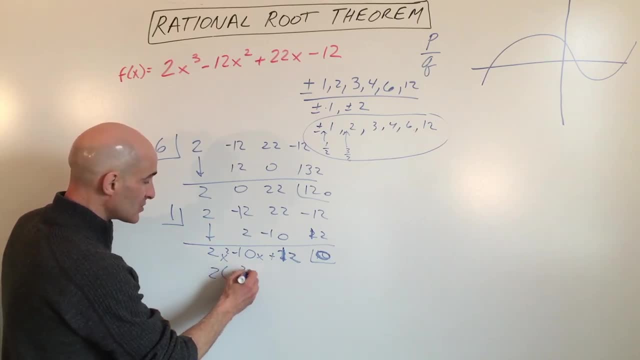 or we can factor. so here I'm just going to factor, I'm going to factor out the 2 and here I can factor this into two binomials: x minus 3 and x minus 2. if I set these factors equal to 0, we get 3 or 2, okay. so we have our zeros 1, 2 and 3, okay, so what that means. 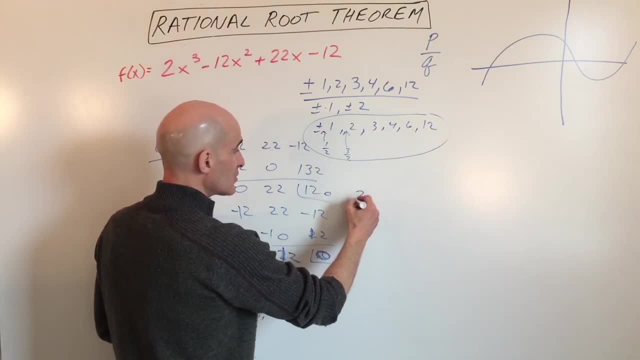 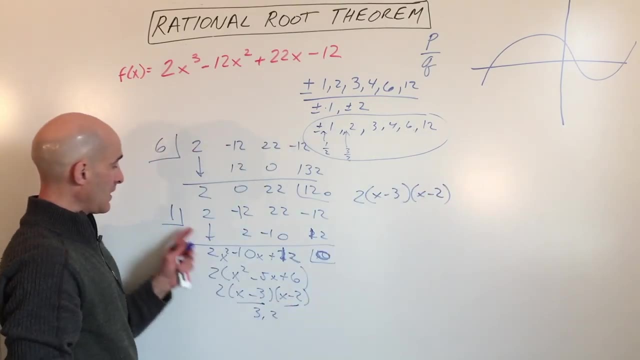 is. you can write this in factored form. it's going to be 2, okay, that's that 2, right there. x minus 3, x minus 2, okay, and then 1 was a 0. so x minus the 0 is a factor, x minus the 0 is a.